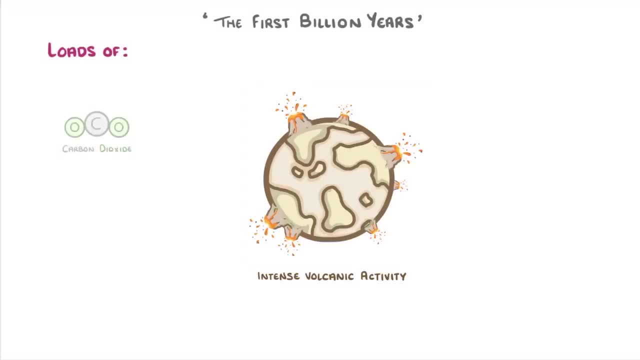 volcanic activity, which produced loads of carbon dioxide, water vapour and nitrogen, along with smaller amounts of methane and ammonia. This meant that the early atmosphere was mostly carbon dioxide, Much like the atmosphere in the first billion years of Earth's history. the atmosphere 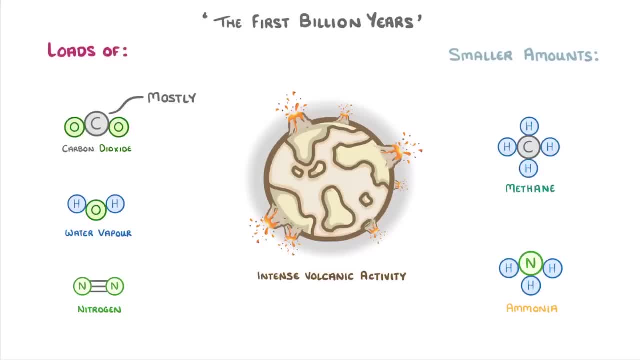 in the first billion years of Mars and Venus. today, As the water vapour condensed into liquid water, though, it formed the oceans, and this allowed lots of the carbon dioxide from the atmosphere to dissolve in them, where it could go on to form carbon precipitates and then finally become sediments in the seabed. 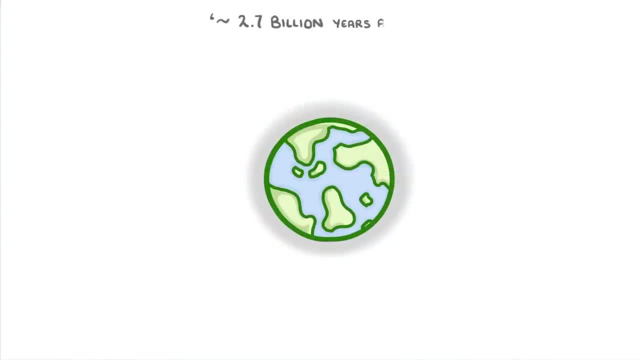 The next major change started about 2.7 billion years ago. Slowly at first As algae began to appear, But becoming more rapid as green plants evolved over the following billion years. This is because both of these groups of organisms are able to photosynthesise. 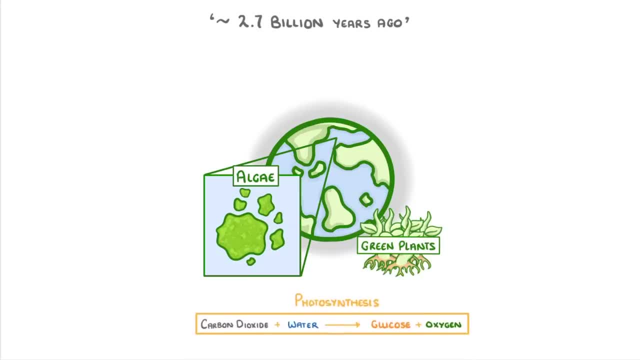 And, as you can see from this equation for photosynthesis, this not only takes in carbon dioxide, but also produces oxygen. So, as algae and plants have photosynthesised over the past couple of billion years, the amount of carbon dioxide in the atmosphere has increased. 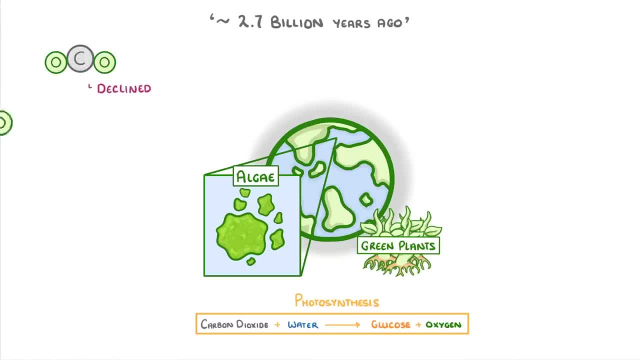 And that's because both of these groups of organisms are able to photosynthesise. The amount of oxygen dioxide in the atmosphere has slowly declined, While oxygen levels have slowly built up, Which eventually allowed more complex life like animals to evolve. Now, algae and green plants could only hold a relatively small amount of carbon in their 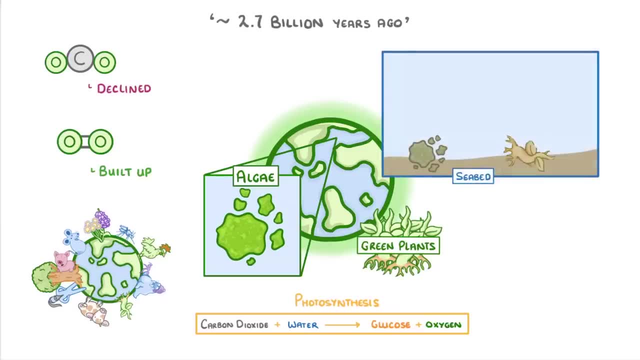 bodies. When they died, though, they fell to the seabed and became buried in layers of sediment, And, over millions of years, this sediment became compressed to form sedimentary rock, oil and gas, which trapped the carbon to stop it from getting back into the atmosphere. 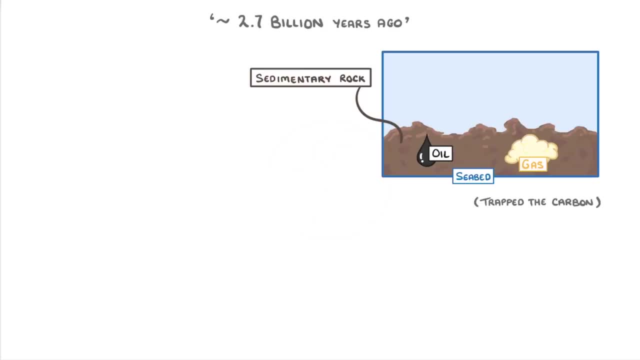 The exact substance that was formed in this process, though, depends on the type of organism being buried and the conditions involved. For example, crude oil and natural gas are formed mainly from dead plankton, which are a diverse group of tiny organisms that float.